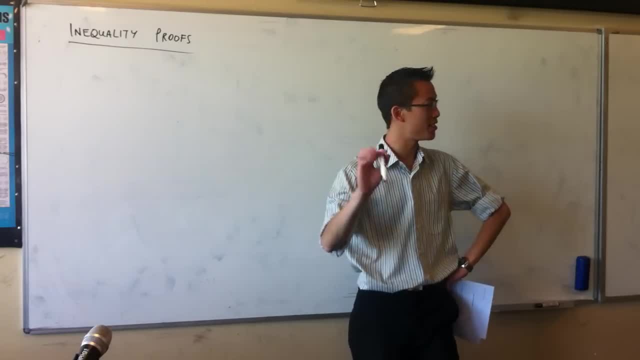 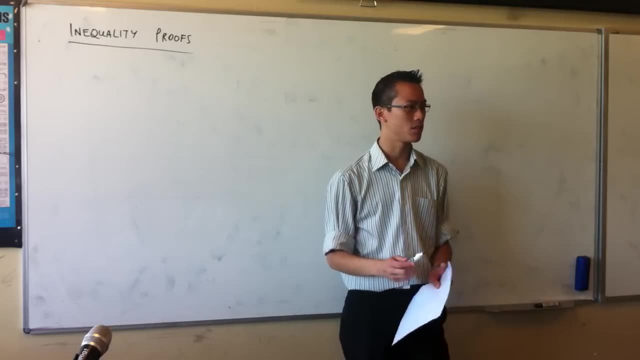 So we've looked at, say, the series. We started off with nice easy series that we know how to deal with. already We looked at some algebraic identities which are a little weirder, but they still weren't that hard to do. 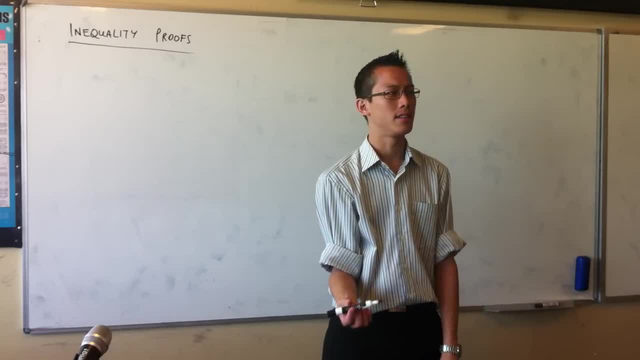 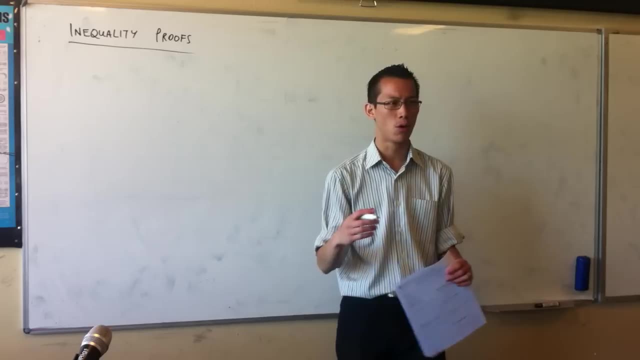 And then what have we been doing? more recently, I'm stuck with factorials in it and divisibility. more recently, I've been going through them in the order where I think they become more complex or more. maybe not more complex, but you have to think harder. 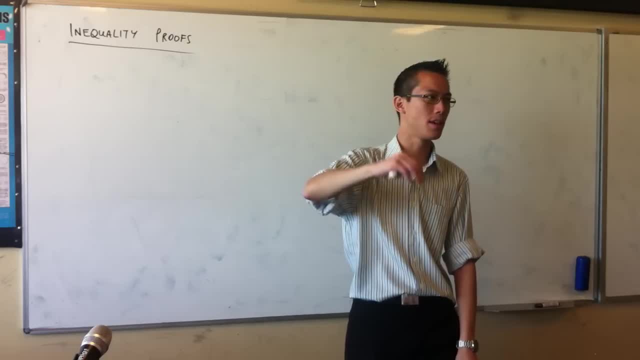 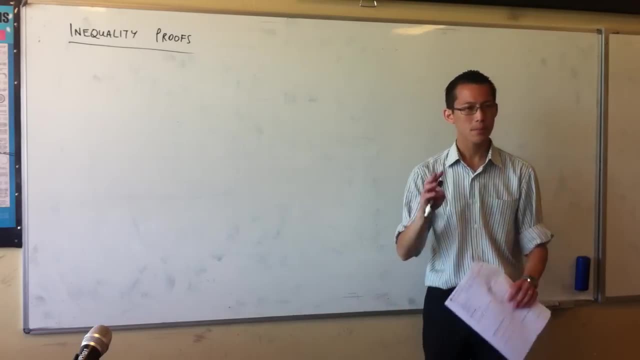 It's less formulaic. You can't just go through the steps and machine it out. You've actually got to think as you're going through it, And I think this is a good example. So, So let's begin. Here's our first one. I think it's three to the air. 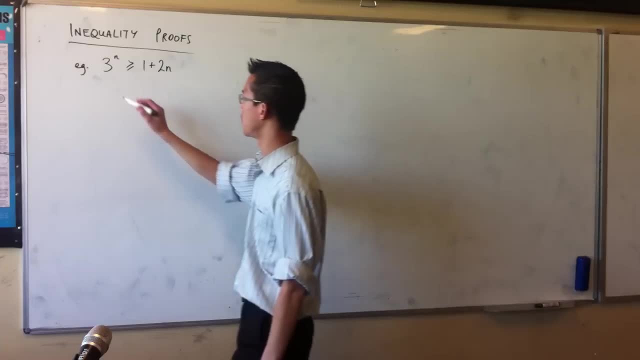 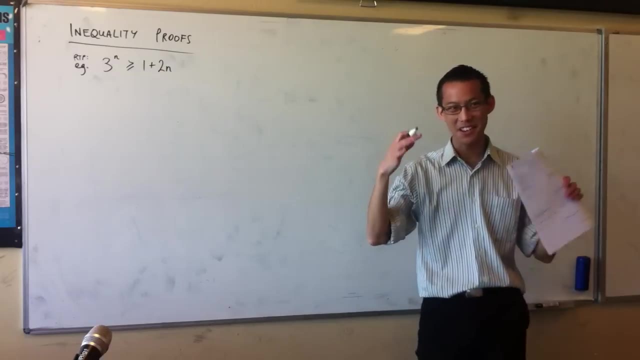 Okay, So this is what we're required to prove. Sorry, Okay, Let's see. Do you know well enough now that I don't have to? Do you know well enough now that I don't have to, to write it down? 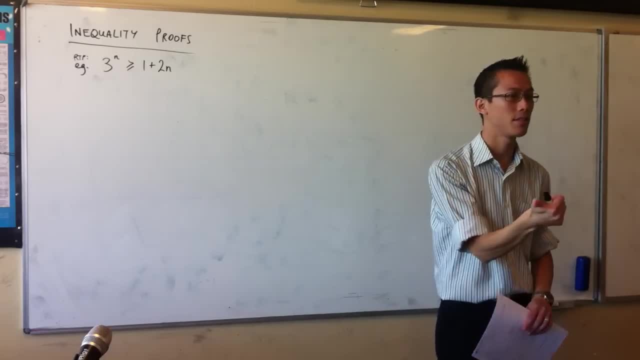 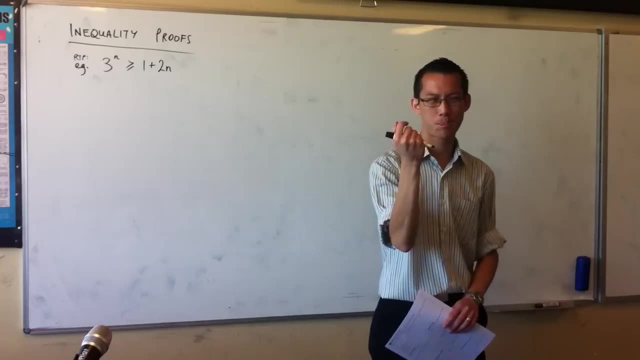 We're at four steps. We want to test for the first allowable value. assume that it's true for a particular value, k. prove that it's true for the next value, if you can assume that it's true for k, and then you just conclude with your explanation. 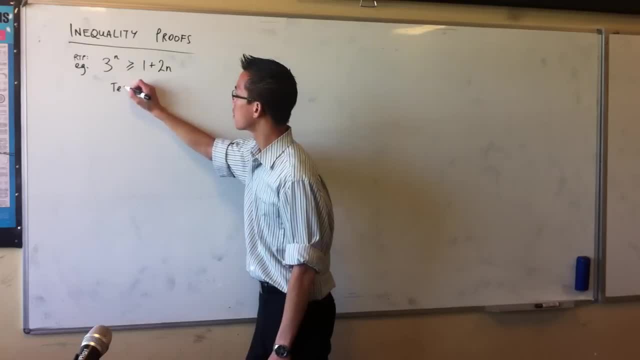 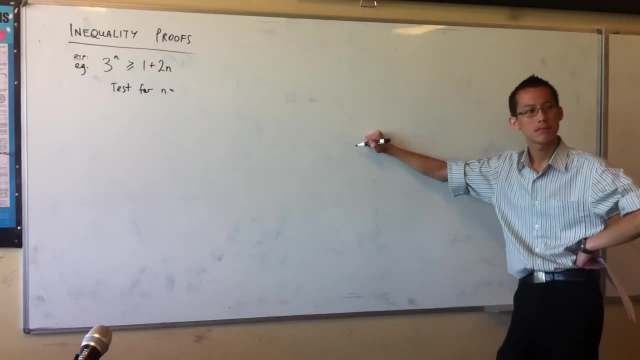 Okay, So let's give it a go, shall we? What is the first allowable value? What do you think? Look at it. I think it works for zero, doesn't it? It doesn't work for, Actually, does it? 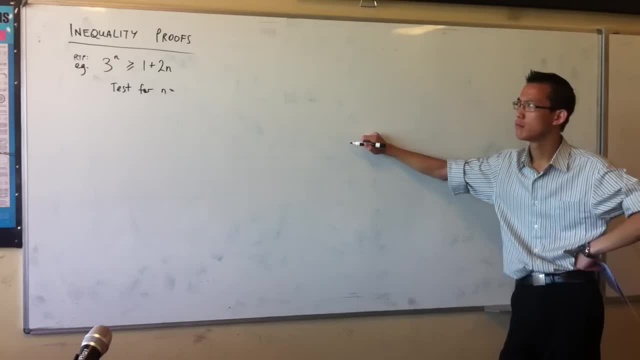 Does it work for negative numbers? It does work for negative numbers. That's interesting. I'm going to start at zero. I didn't specify, but usually it will be zero and on if you can get zero Right. So zero is kind of like the best case, but sometimes it breaks things down. 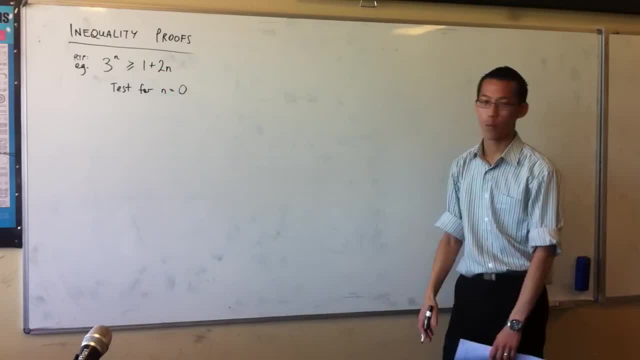 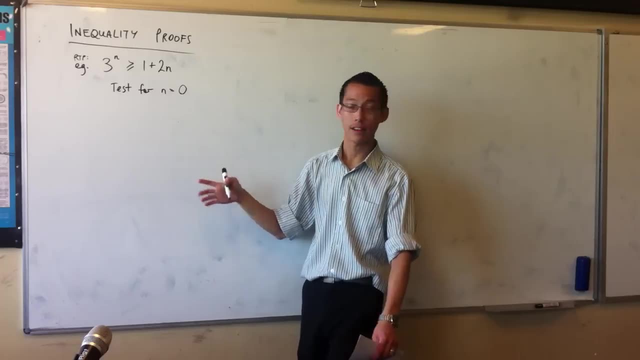 Because we have that equality in the inequality, we can use zero, okay, So let's give it a go Now. usually you start off by saying left-hand side equals this and the right-hand side equals this, and that's fine, okay. 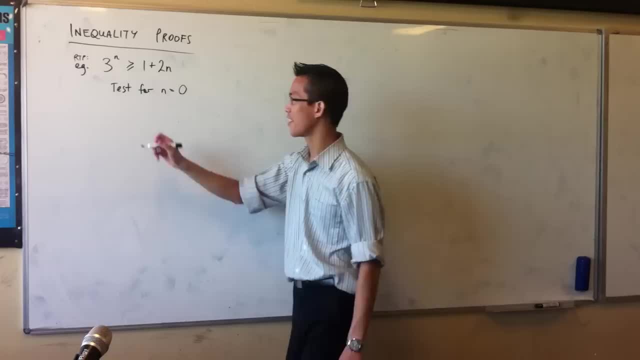 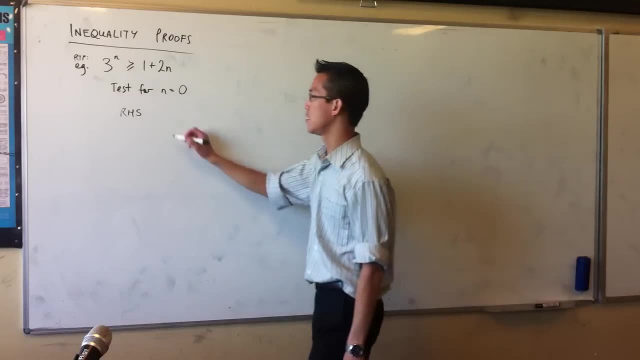 For inequalities. I'm going to start with the right-hand side. Hopefully it will become clear in a second why, even though that might seem backwards to you at first. okay, The right-hand side is equal to one plus two, lots of zero, which is one, okay. 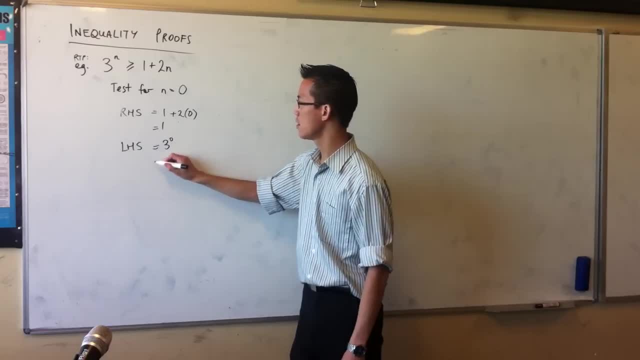 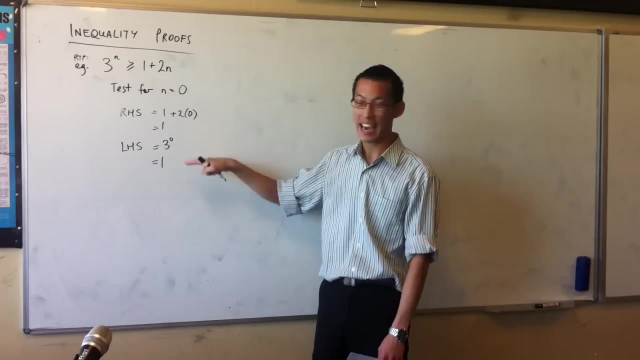 So now I can look at the left-hand side, which is three to the power of zero, which is one. And now what do I do here? I don't say it equals the right-hand side, even though in this case it actually does right. 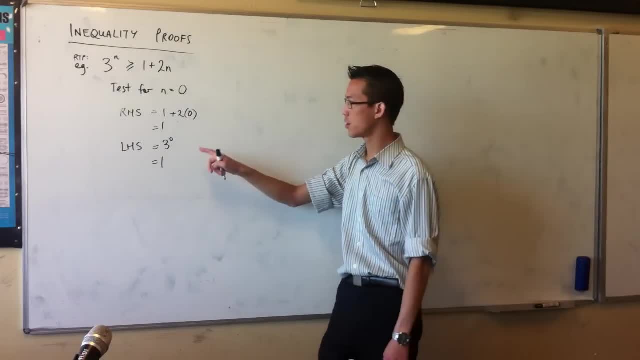 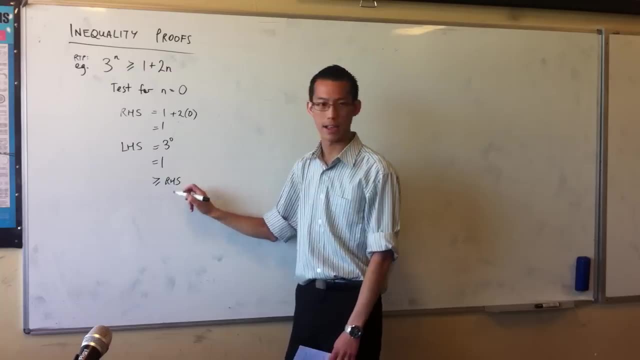 These numbers could be different, and it would still satisfy the statement, right? So instead I'm going to take my inequality from here, right? So I'll say one: right? Well, that is greater than or equal to the right-hand side, and it does satisfy it, right? 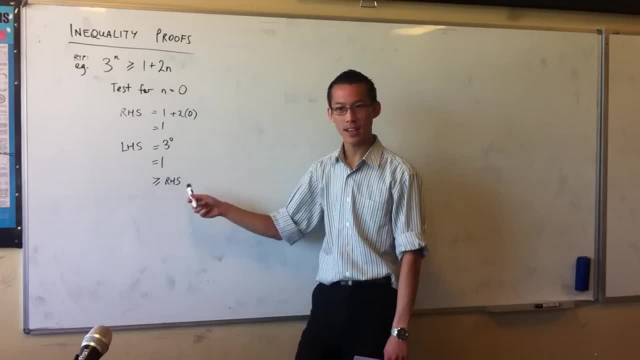 Can you see why I did the right-hand side first now? Because now this final statement here is: the left is on the left and the right is on the right. okay, If you did the left-hand side first, you're going to have 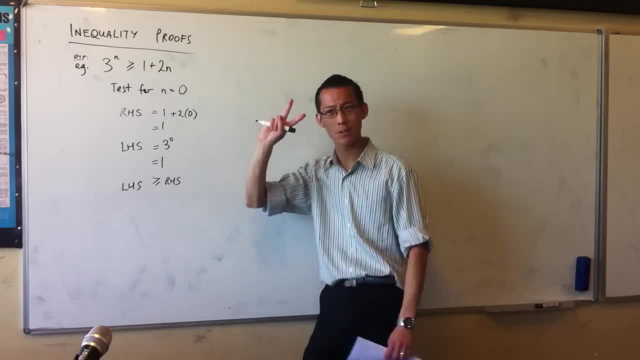 right-hand side here, and you'll be like right-hand side, left-hand side, and your inequality will be backwards and it's. this is confusing. Just have it left on the left, right on the right. okay, There's the test. 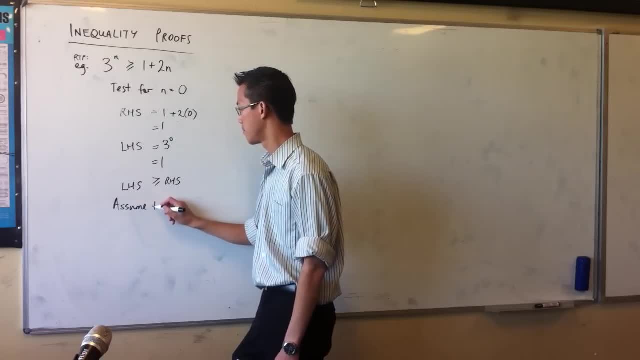 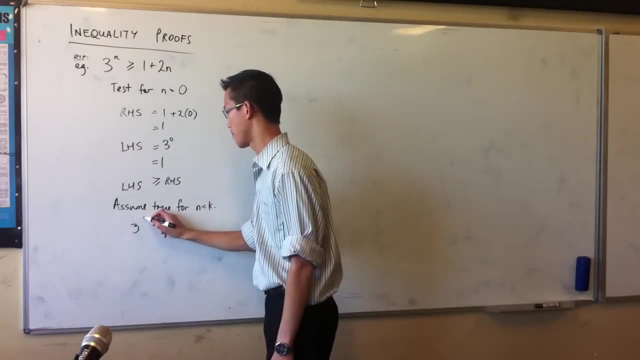 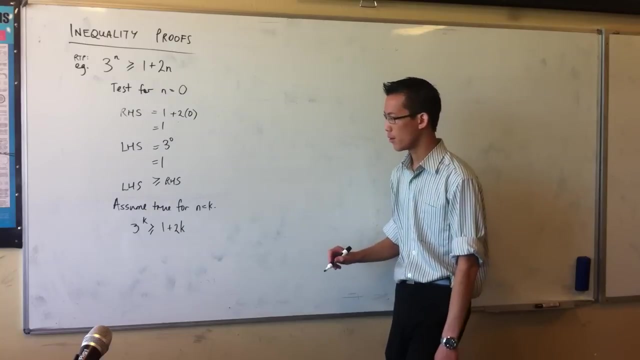 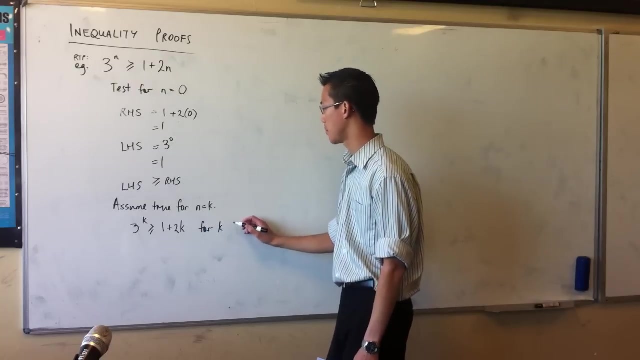 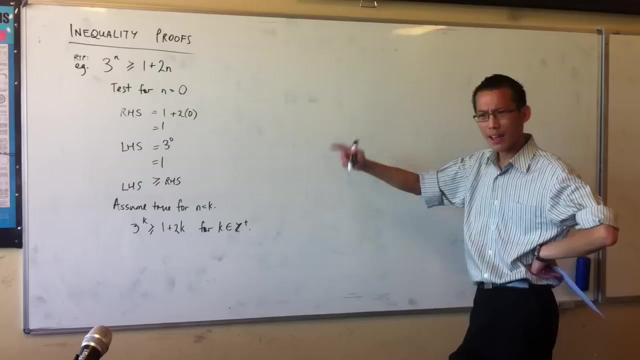 Now we assume. So just straight substitution, okay. Also, don't forget to mention what k is right. So I guess we'd say k must be a positive integer. Like we just noticed, I think it does work for negatives. 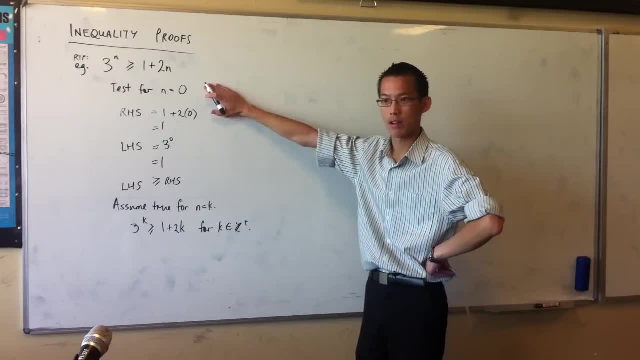 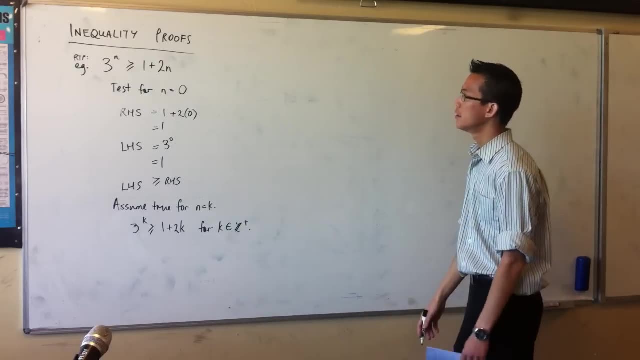 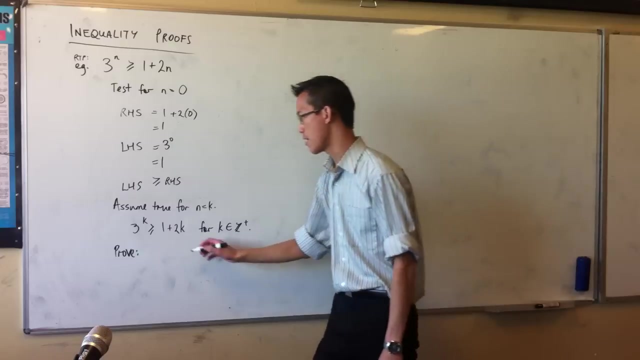 But for now, since I'm starting from zero and I'm going to go all the way forward, I'm just going to say: k can be anything forward from zero. okay, All right. so now my proof. okay, Proof. What am I required to prove for k plus 1, right? 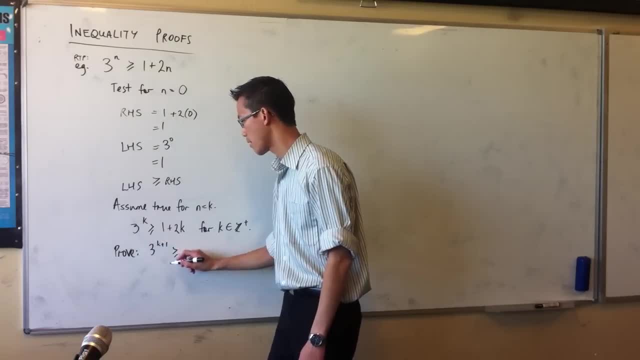 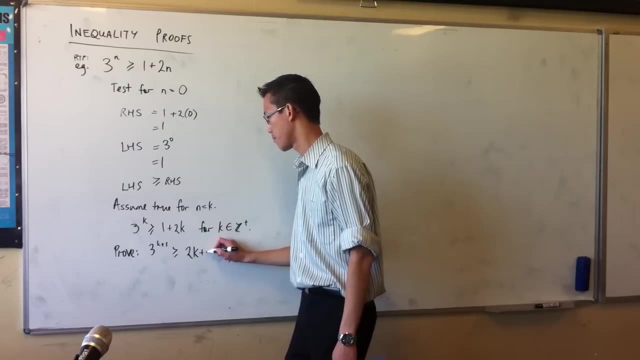 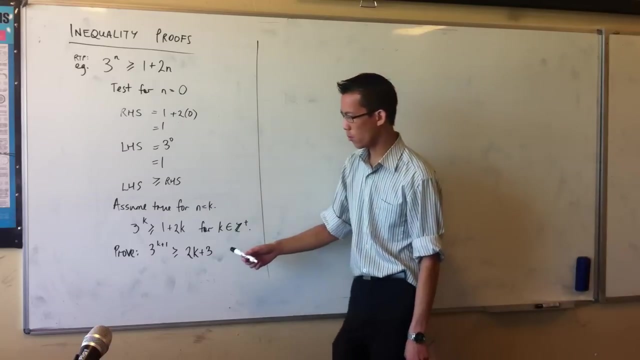 So I've got 3 to the power of k plus 1, should be greater than or equal to. this is going to be 2k plus 3, right, Okay Now, usually when we've been proving these, 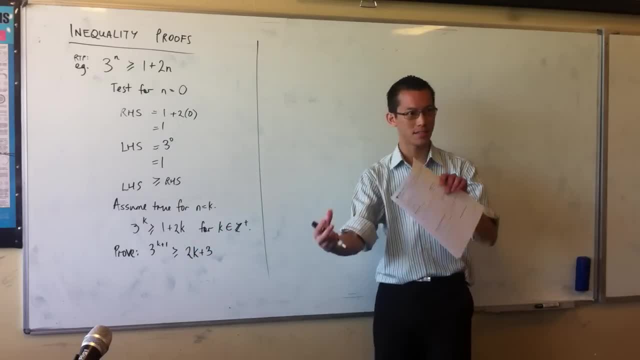 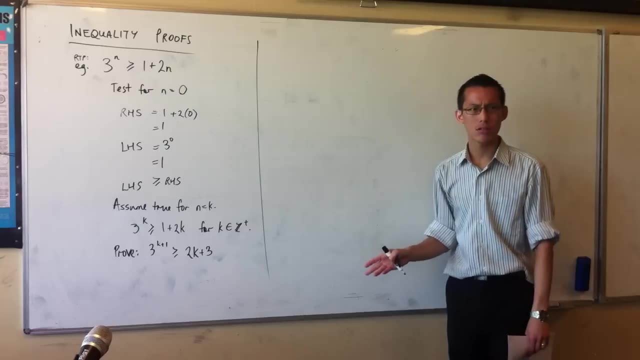 you sort of start with this line and then you sort of twist it and manipulate it around until you can get something which will let you sub in your assumption. okay, I think you can do that, but with inequalities I think it will feel more logical if you actually start. 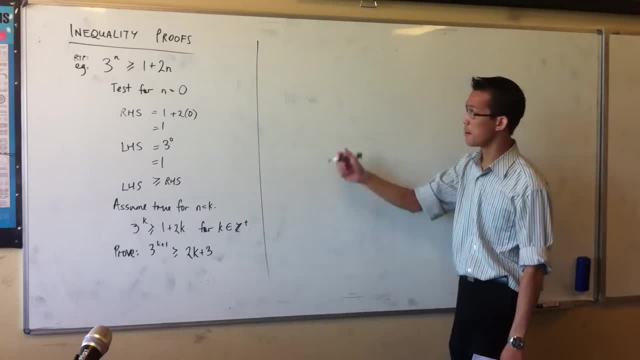 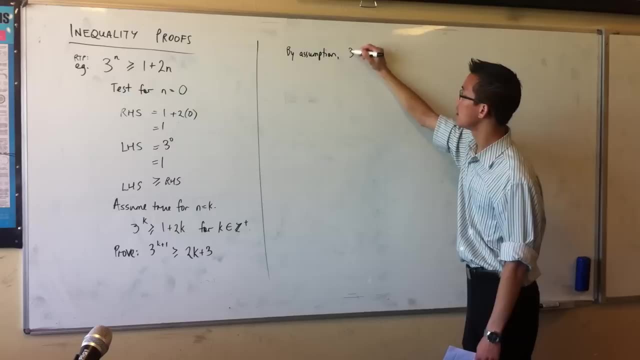 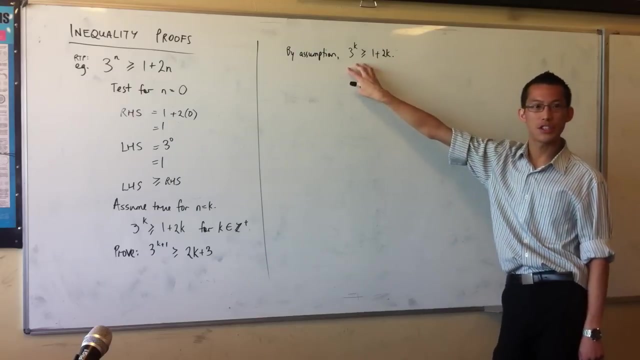 with your assumption as your very first line. okay, So I'm going to say, by assumption right at the beginning, 3 to the k is greater than or equal to 1 plus 2k. okay, And now I'm going to try and twist and turn this to get into my proof. okay, 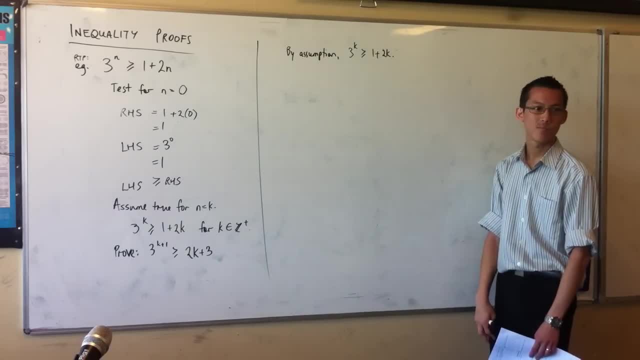 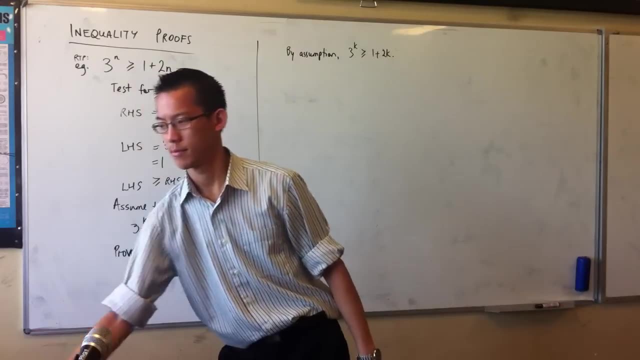 So what do you think is the easiest thing? Okay, First step. what do I want to do? What's the most natural thing to get from this line to that one? You could go with either side, right? I haven't tried the right-hand side. 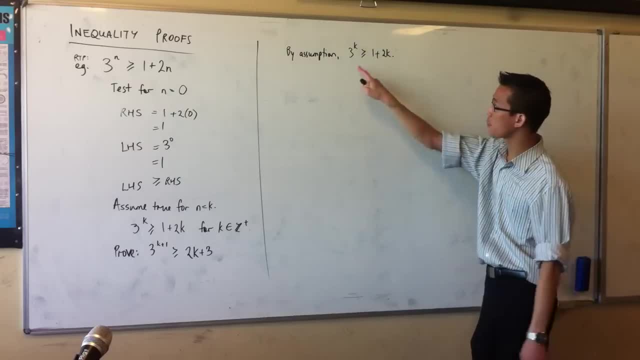 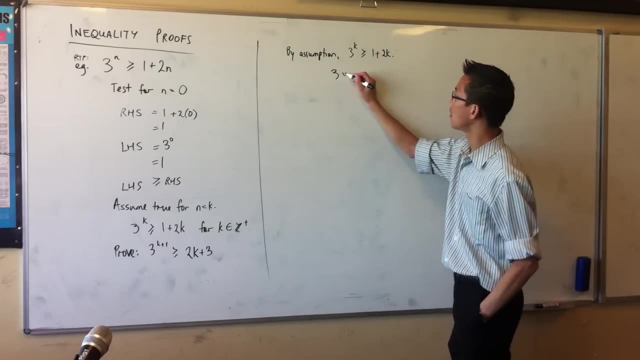 so I went for the left straight away, maybe because I see the left first. So to get from here to here I have to multiply by 3, right, That's what the plus 1 is okay, So I'll multiply by 3.. 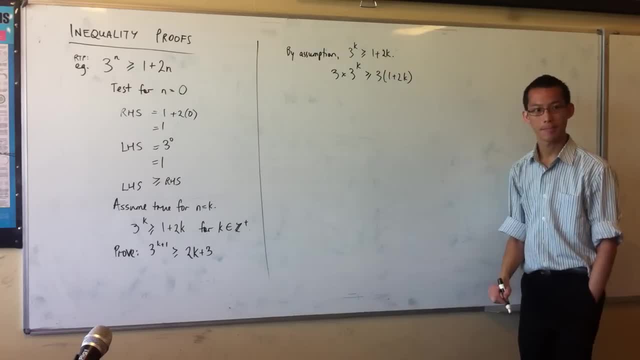 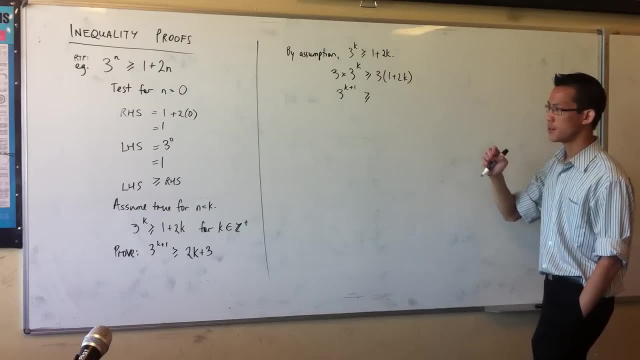 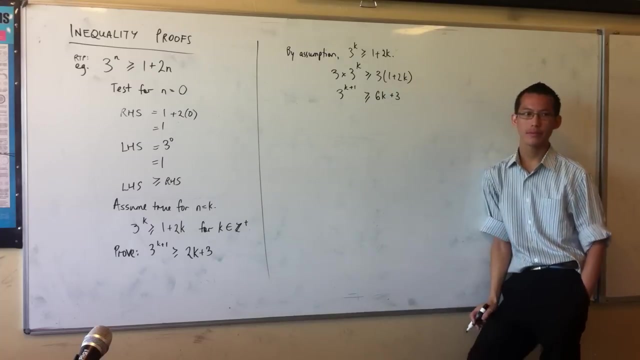 So I've got to multiply this side. multiply this side by 3 also. okay, Now I've got my left-hand side. nice Now over here. hmm, let me just switch the order around a little bit. I've got 6k plus 3, okay. 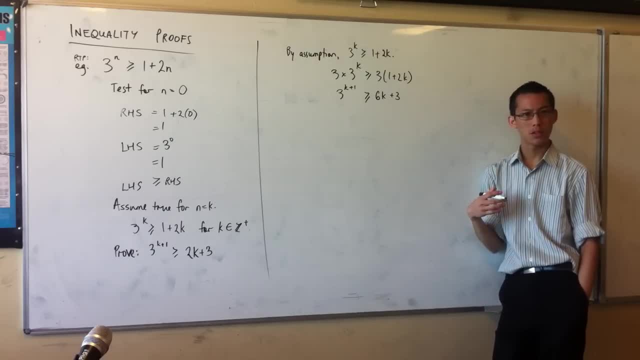 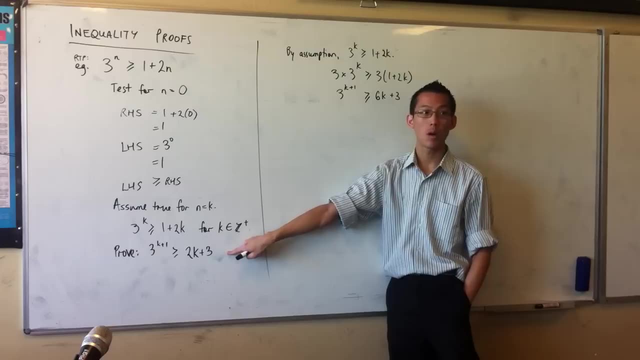 Now here's where I mean that inequalities will force you to just think a little more. okay, This is not that. It's not what we were setting out to prove. At least, it wasn't exactly right, But it's enough, isn't it? 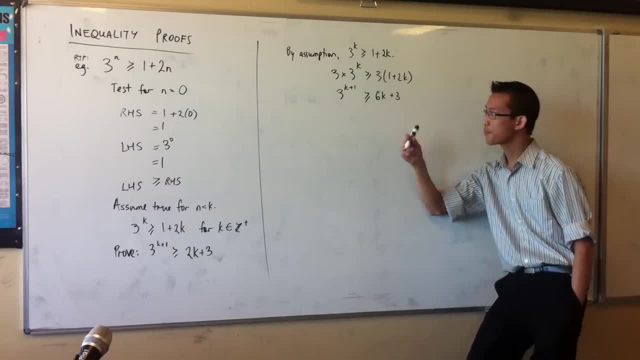 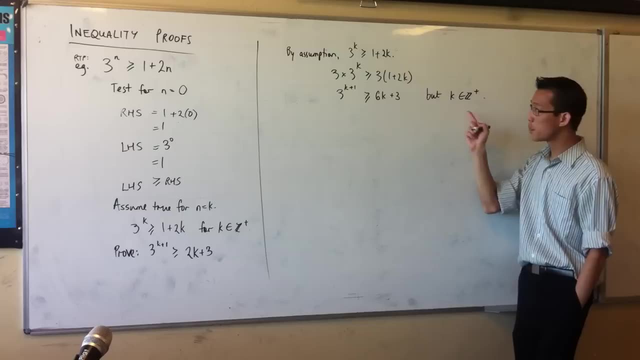 Hmm, can you see what's happening? Um k, right k, excuse me, is a positive integer, At least that's the way I've specified it, right? So if it's positive, then surely 6k will be bigger than 2k, yeah. 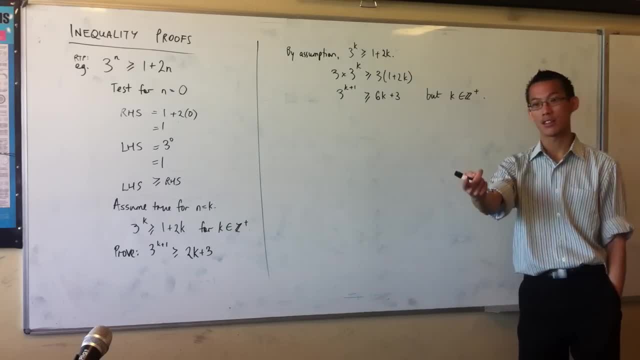 6k is bigger than 2k. I hope right. Um, so there you go. there's a reason why k as a negative won't work, for at least this method of proof. okay Now, 6k is bigger than 2k. 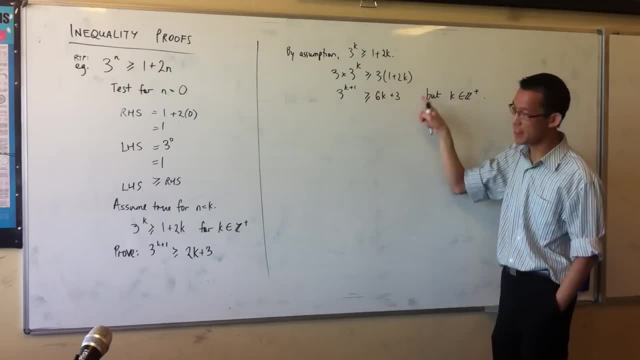 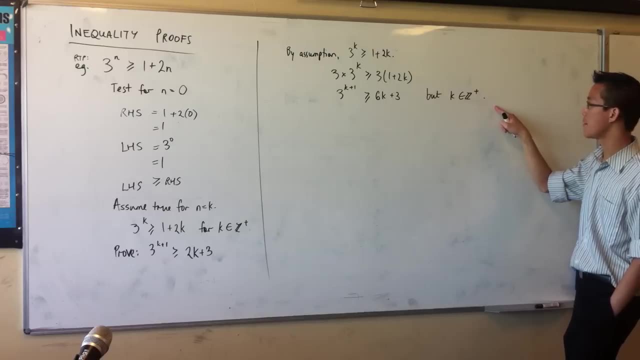 and 3 to the power of 2k. 3 to the k plus 1 is bigger than that right. So surely 3 to the k plus 1 must also be bigger than this right. So I would say, since k is positive right. 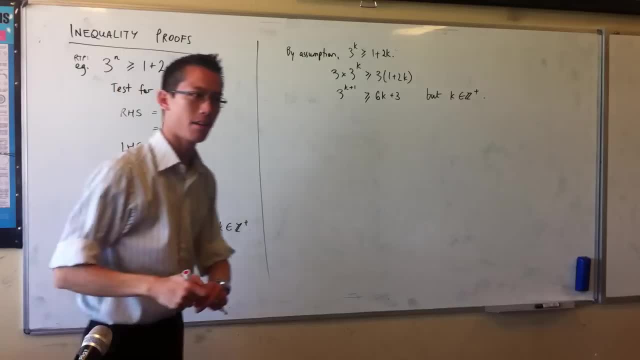 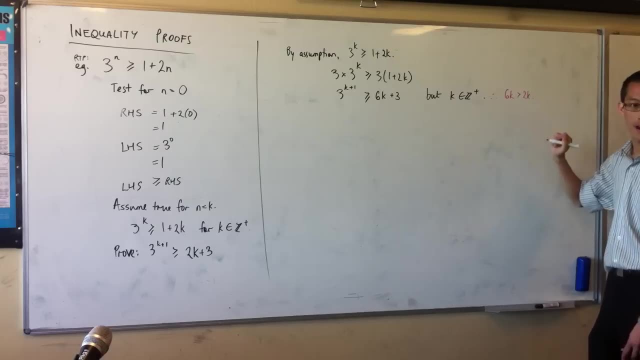 Um, you can put on the side here. I don't think this bit is necessary, but it's helpful for your logic, I think. Um, therefore, 6k is greater than 2k, right? So I'm just making the connection between what I have. 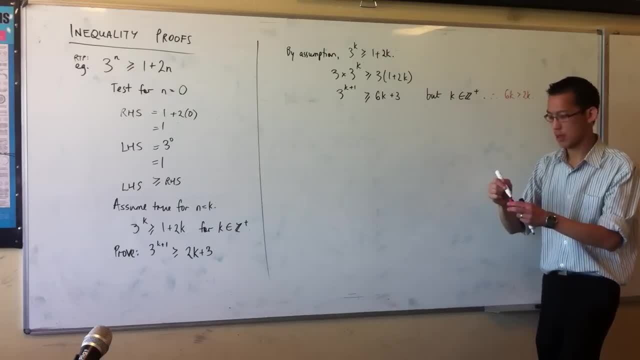 and what I have in my um, what I need to prove. okay, So, seeing as 6k is greater than 2k, um, because this is an integer, this is an inequality. I can just shift things around, right. 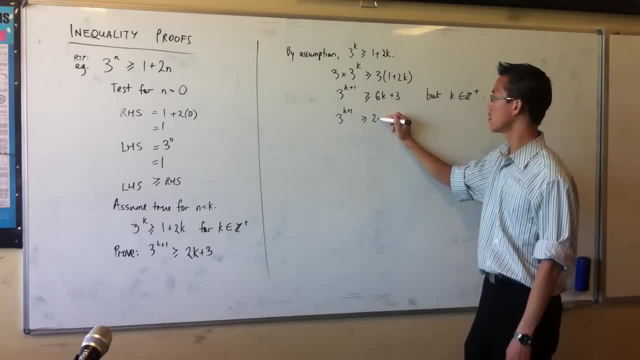 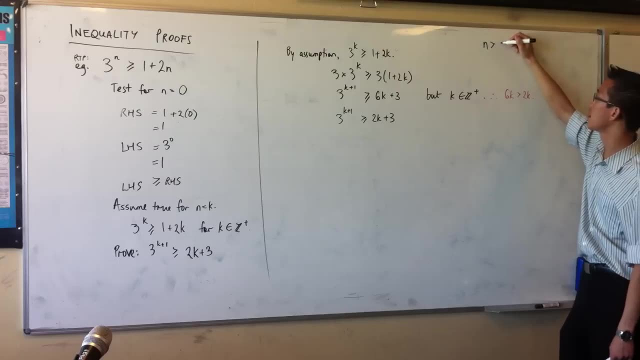 I can say: 3k plus 1 is greater than 2k plus 3.. This implies this, right? It's just like saying: if a number is greater than 10, then surely it's also greater than 5.. That's all I'm doing, okay. 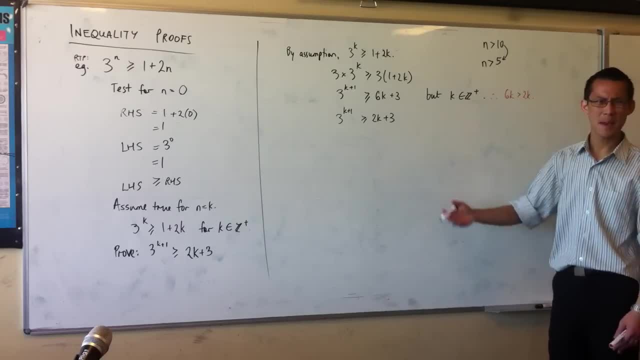 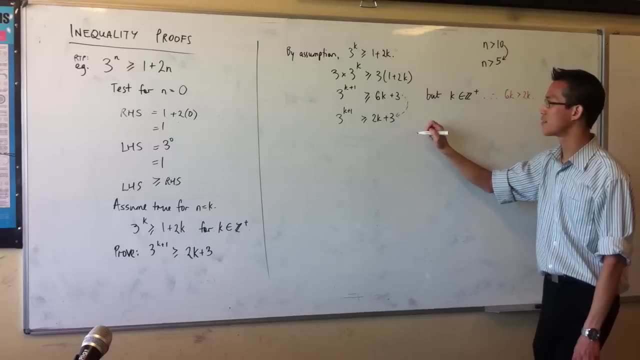 This implies that And that's it okay. Now, maybe you didn't think that was that hard, maybe you thought that was very obvious, okay, But I know, when I was getting through this topic myself, um, going from here to here is kind of. 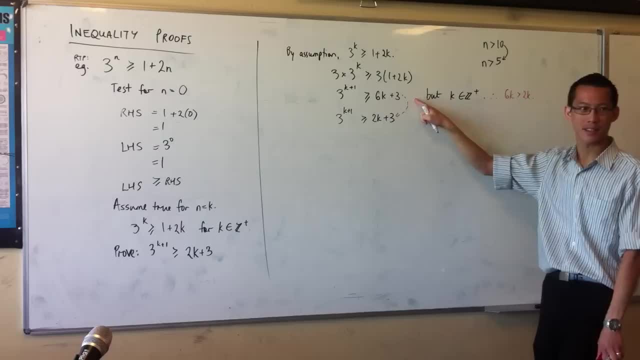 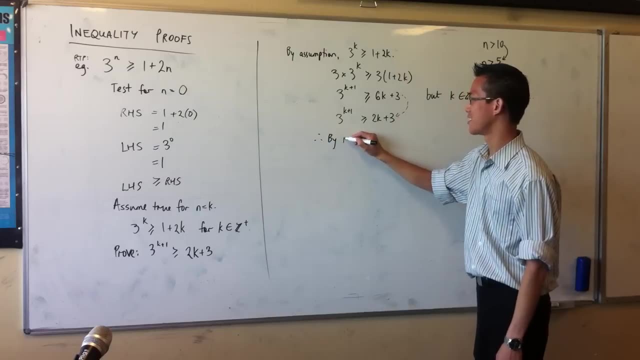 when you get to this point, you think, huh, I just want to get there. Um, well, that is there. okay, That's it. It's very short, Okay. Um so, by the principle of mathematical induction, I'm on my last step now. 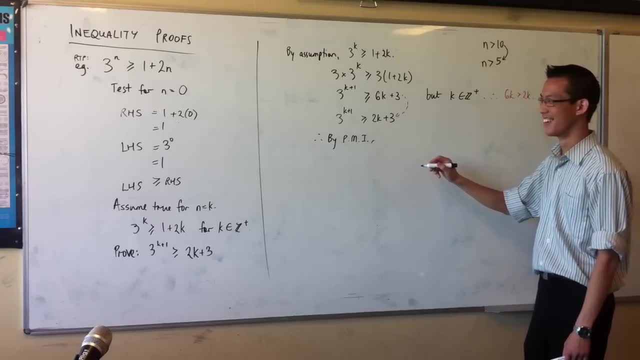 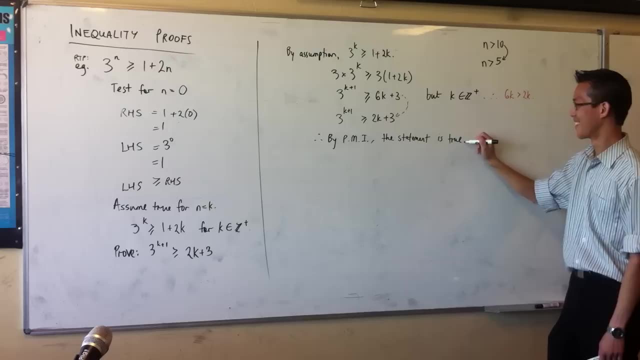 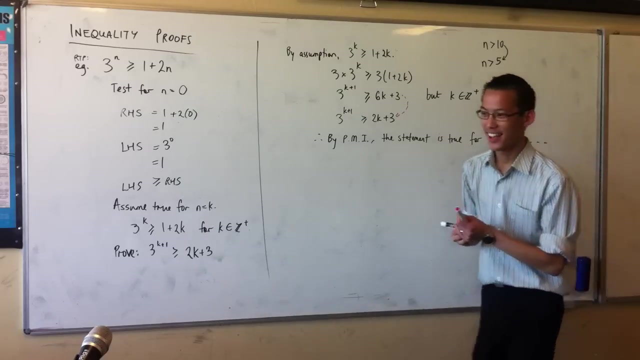 Introducing Mr Wu. Edit that, sir. Ah, report card F. Report card F. Uh, zero, sorry, I have nothing to add. Okay, Done, All right, Okay, So, um, that seems okay. 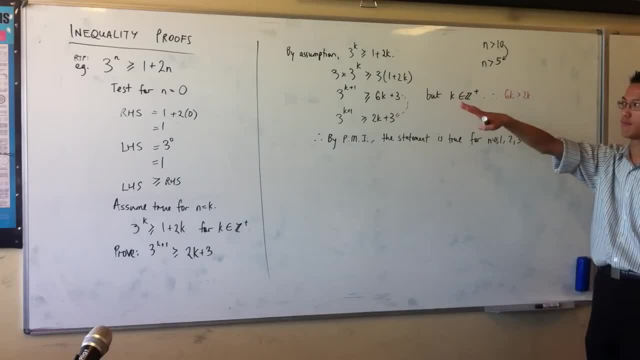 Let's. let's have a go at another one, briefly, which instead of It's, it's got tricky numbers in there, okay. So instead of just um multiplication, which is very easy to deal with, okay, Let's throw a factorial in there. 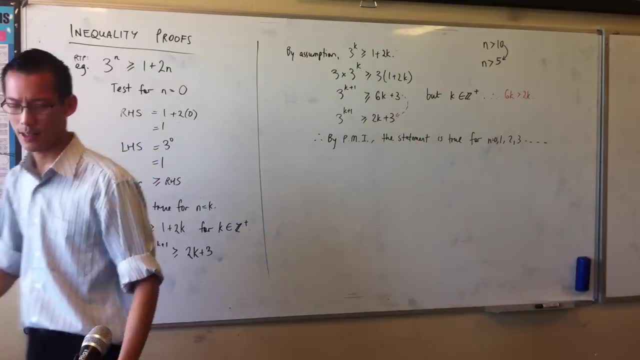 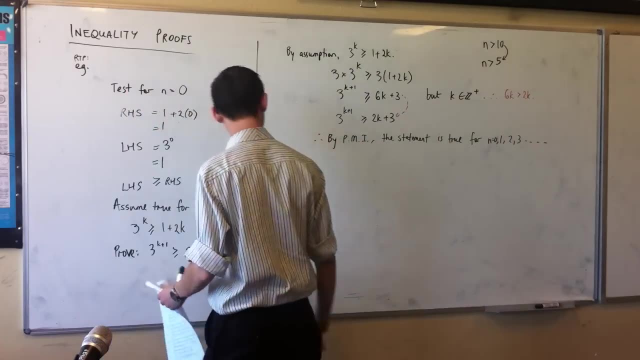 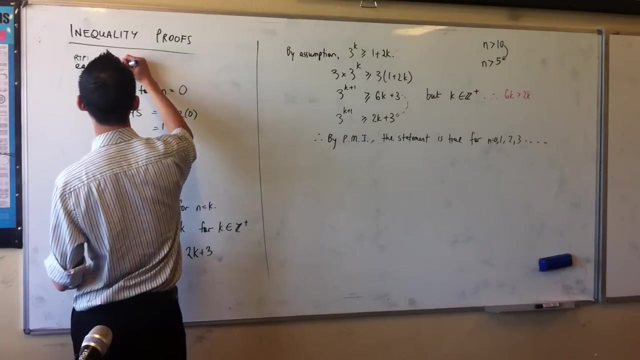 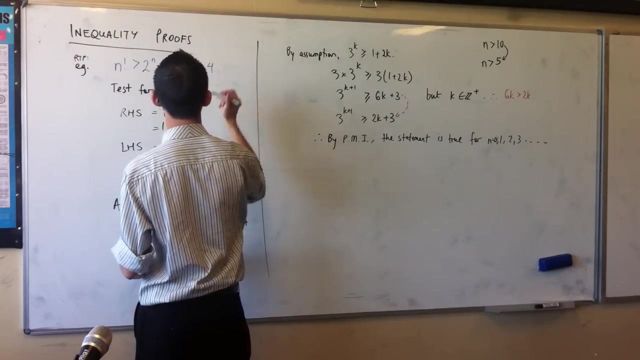 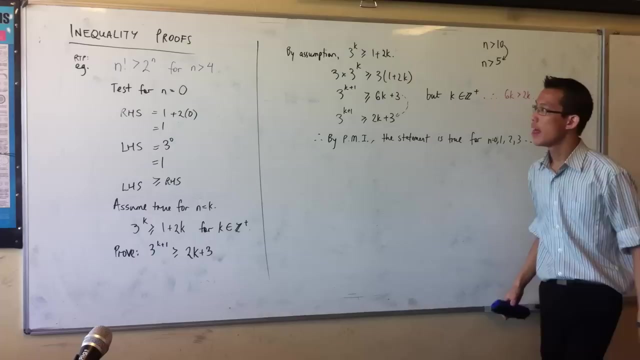 Let's see what happens, okay. So let's um. Oh, it's over here, sorry, Let's do it in a new color, Okay, Uh, I think I mentioned before, right, That a lot of these more um advanced inequality proofs, right. 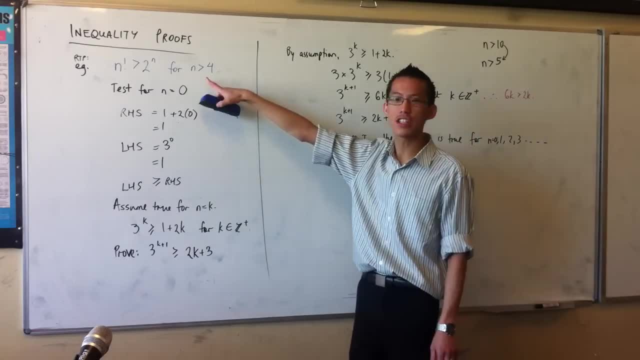 They will not work for zero, one, two, three, four, five and two. No, no, no Right, They will actually only start working at quite large values. okay, So here's an example. right, Therefore? my first allowable value. 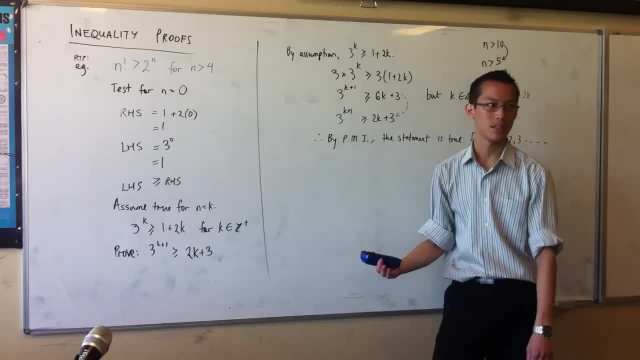 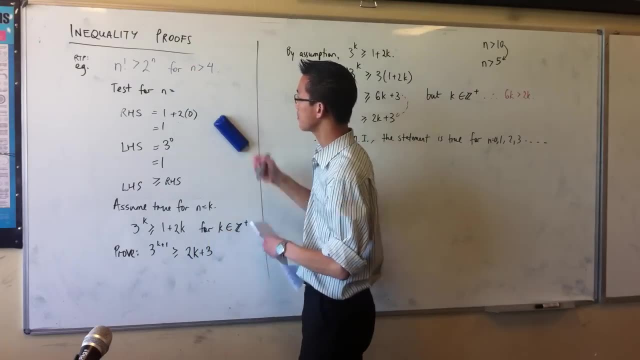 you actually have to use your brain to figure out this. one is five because I'm still dealing with integers. right Induction deals with integers. So instead of n equals zero, I'm going to start with five. Okay, Now again, because of the way the inequality is going to work out. 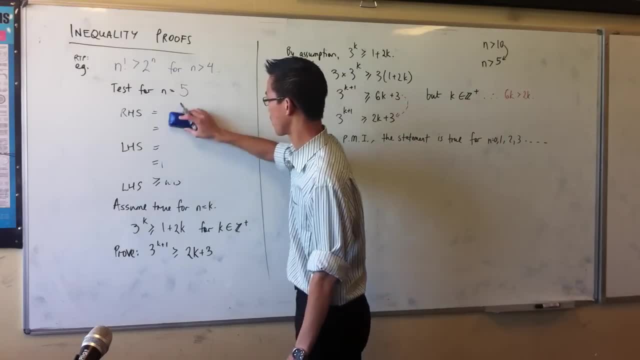 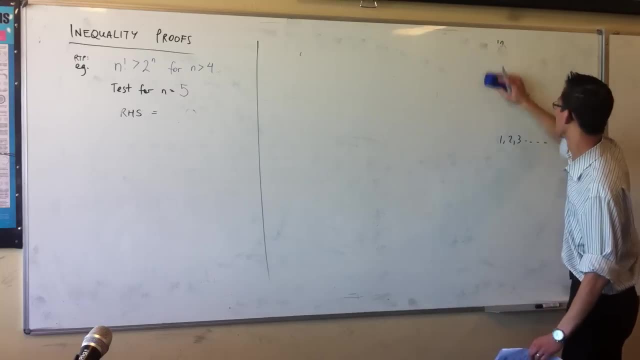 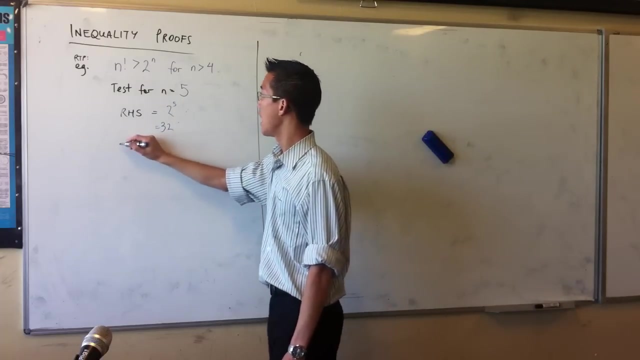 um, I'm going to start with the right hand side, So I'm just going to get rid of all this, Okay. Okay, The right hand side is two to the five, which is thirty-two, And the left hand side is five factorial, which is a hundred and twenty. 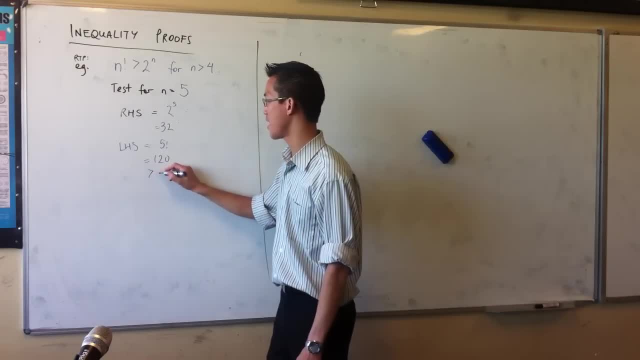 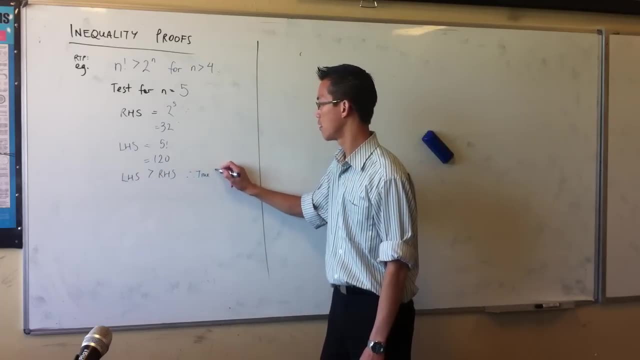 Okay, And a hundred and twenty is greater than the right hand side, the thirty-two that we got before. Therefore, the left hand side is greater than the right hand side, So it's true for the first allowable case. Okay, That was the test. 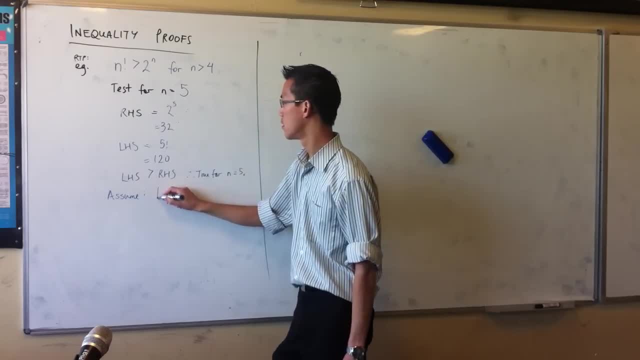 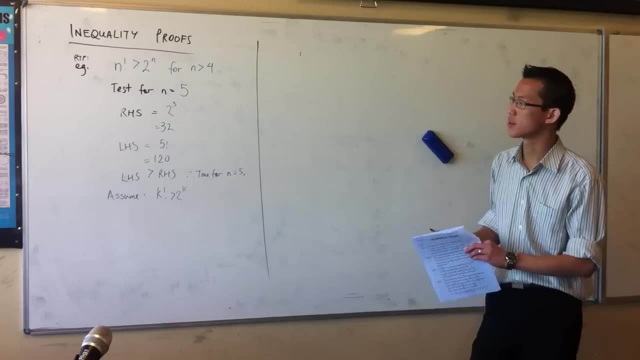 Here's the assumption Now, by the way: because n has to follow certain rules right, Namely it's greater than four Um and k is a particular kind of n, then k has to obey the same rules as well. 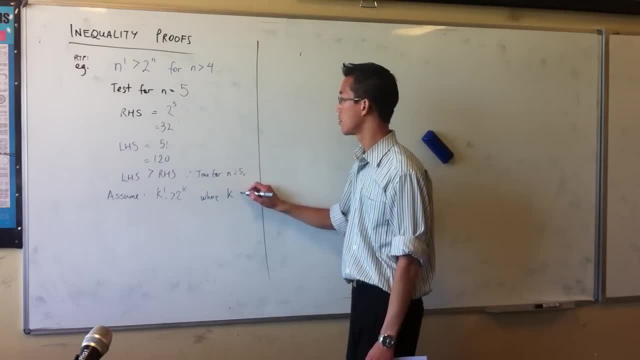 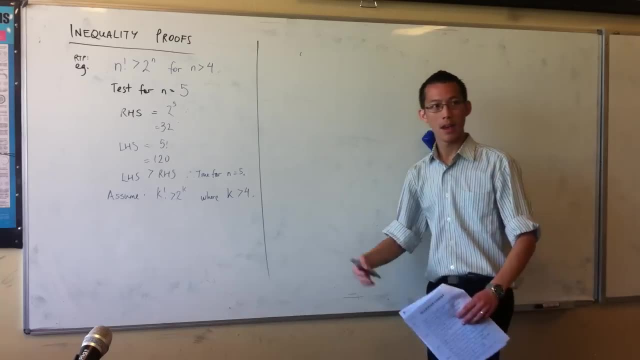 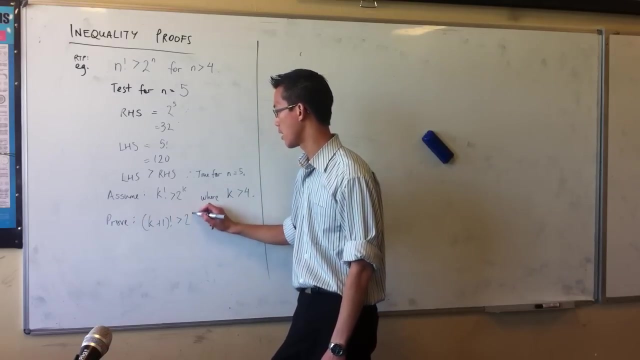 Right, So k? um must be greater than four. Okay, and this will turn out to be crucial for us later on, Later on. Okay, Excuse me Now. what do we have to prove? k plus one factorial greater than. 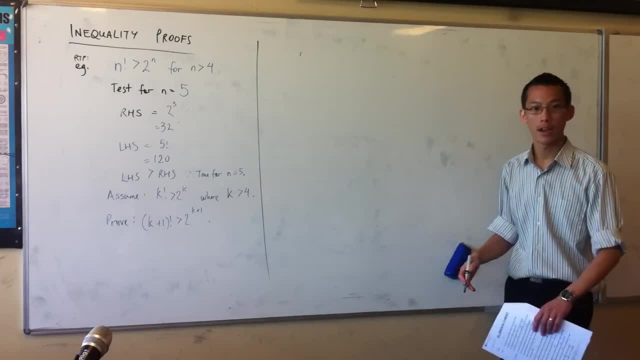 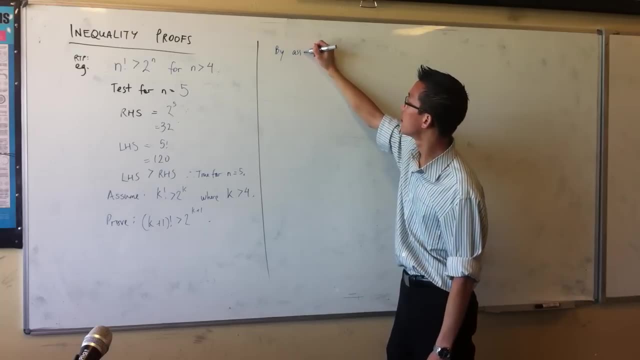 Okay, Now again with these inequalities, I think the easiest way to um, the most logical way to get to the um n, is to actually start with your assumption. So by assumption k factorial greater than two to the k. 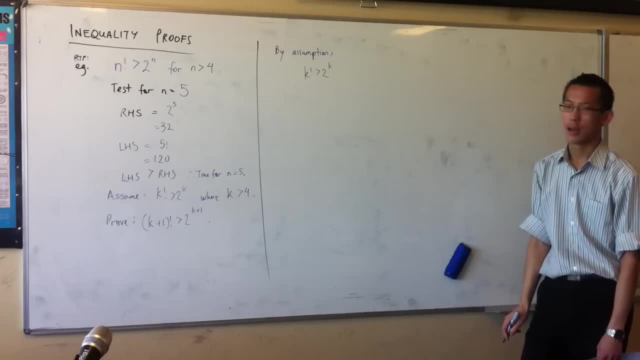 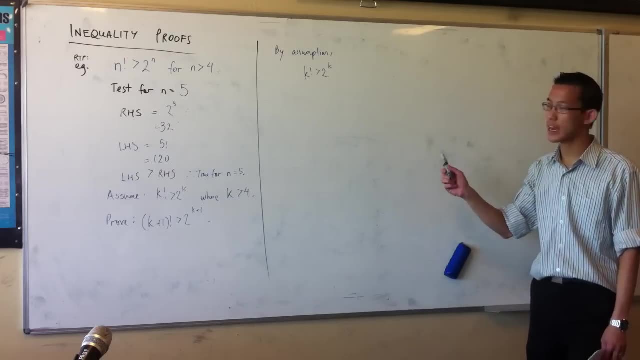 Okay, Now, excuse me, where do you go from there? Um, like I said before, you could go for either side. In this case, I think the left-hand side, conveniently, is still the easiest to go with. Okay. 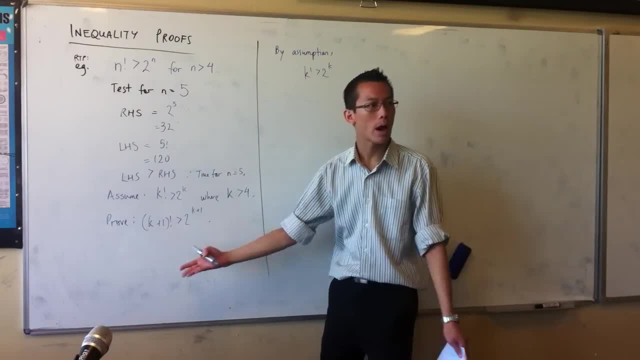 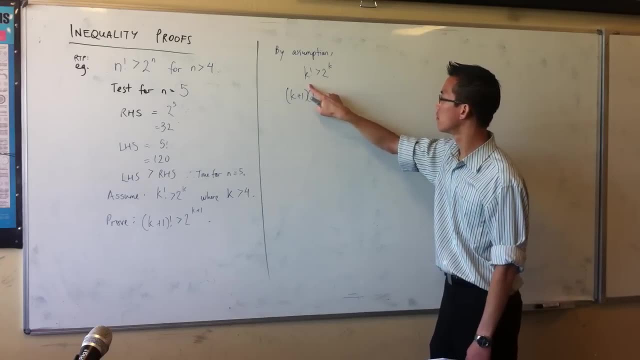 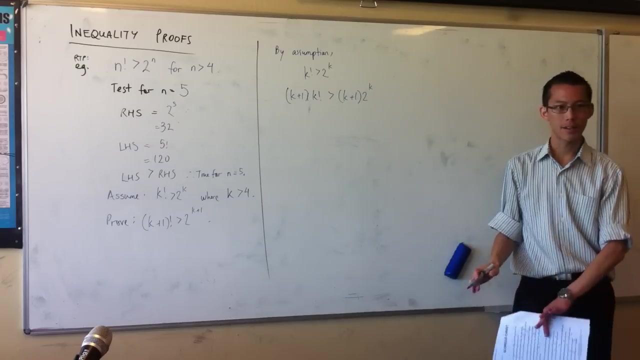 So if I want to turn k factorial into k plus one factorial, what do I have to multiply by? Yeah, just the next one at the end right. Multiply both sides. Okay, Now, on the left-hand side, I'm set. 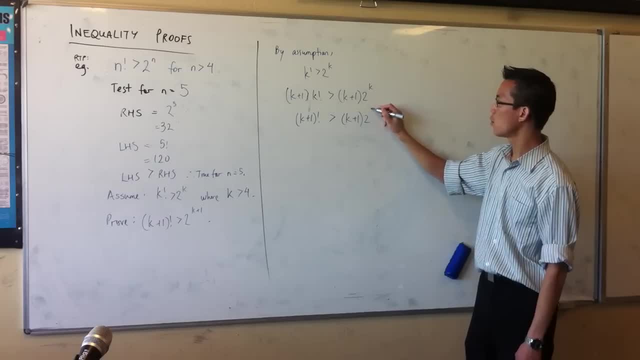 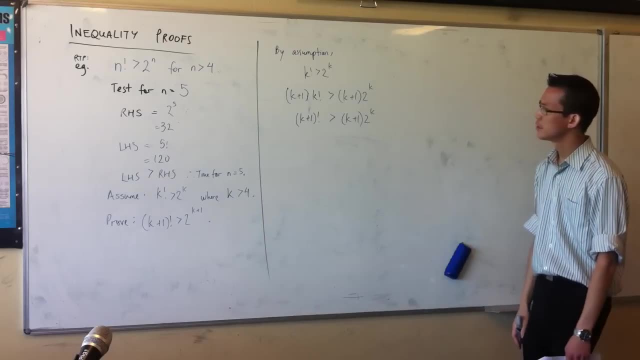 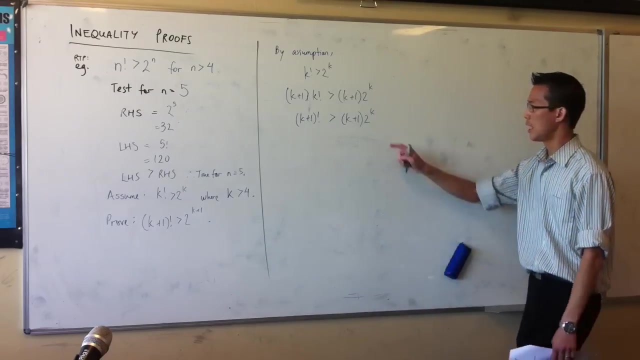 But on the right-hand side, you look at what you've got and you look at what you're supposed to have. Hmm, Hmm Now, um, what's the difference between two to the k plus one and two to the k? 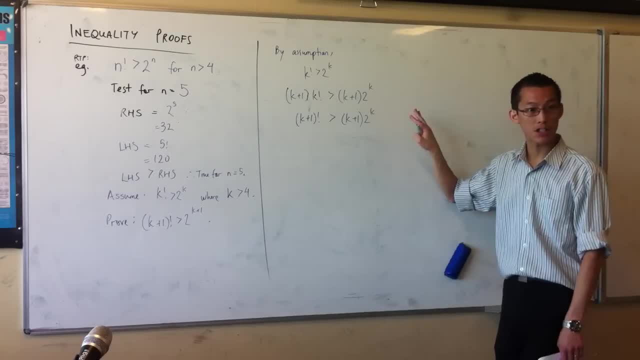 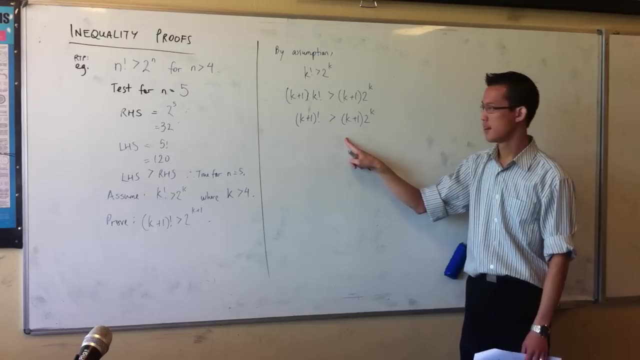 They're different by a factor of two, right? So if I could multiply this by two, I'd get what I want. right Now I'm multiplying by something. I'm multiplying by k plus one Now, just like in the previous question. 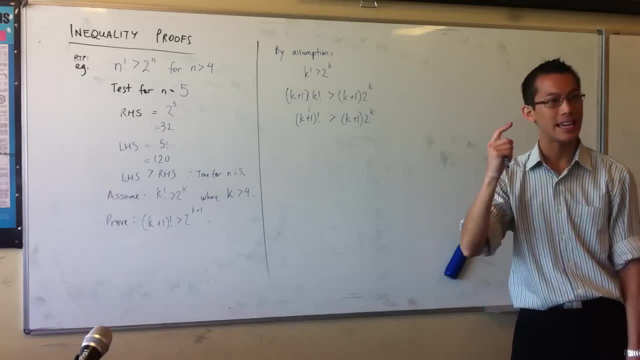 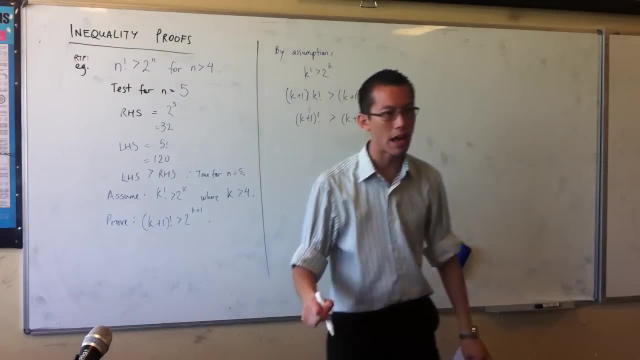 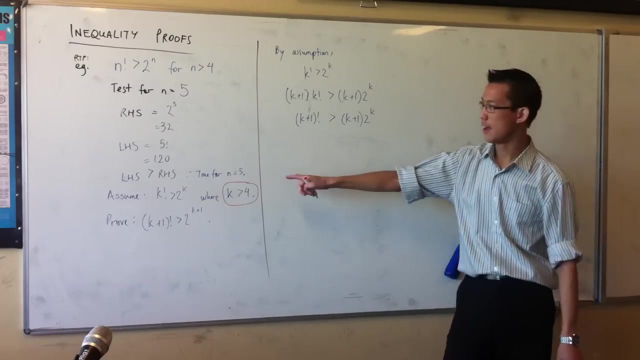 multiplying by k plus one is not just multiplying by two. Actually, it's better than multiplying by two, isn't it? Because if you're multiplying by k plus one, then you're multiplying by at least five. See it Right, That's the smallest value that it can take. 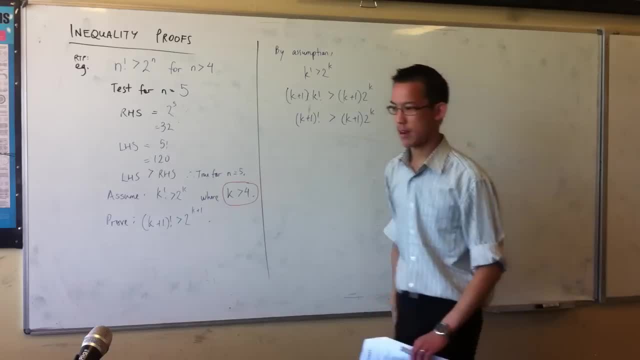 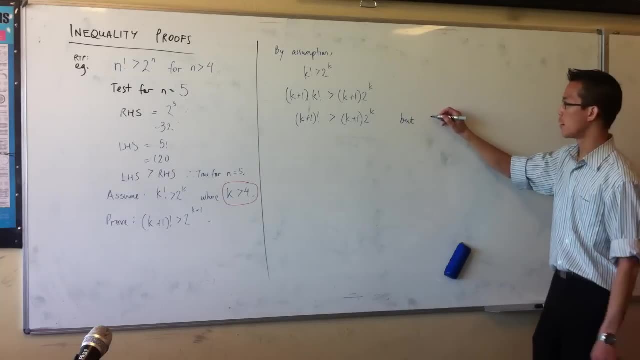 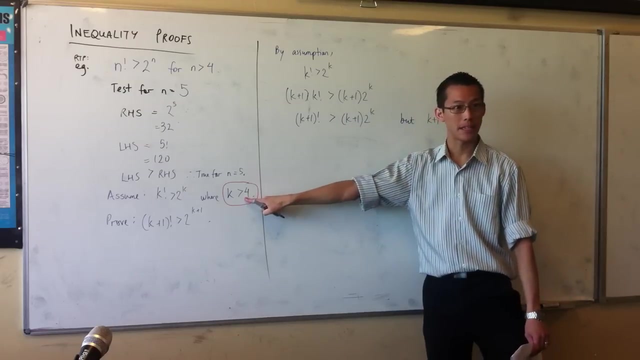 and that's why we um, that's why we tested it Right. So therefore, right, I can say, but right, um k plus one. this thing that I've gotten here, right, um, I could say it's greater than five from here. 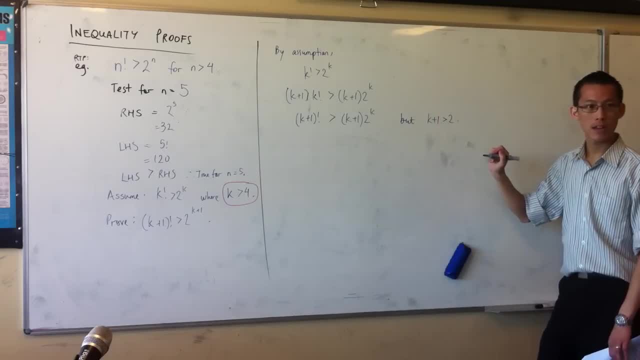 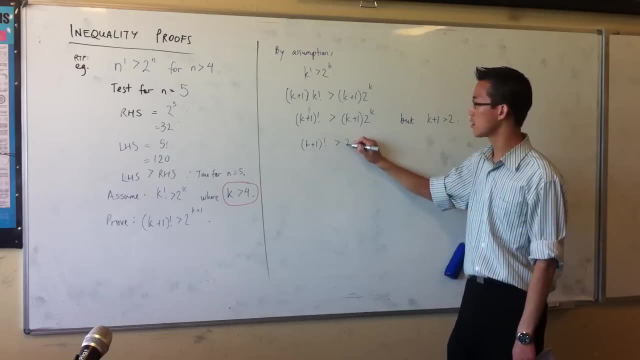 but all I really need is that it's greater than two, Right, Because I'm going to substitute that for a two, So k plus one is greater than two times two. to the k: Again, people seem uncomfortable about this. 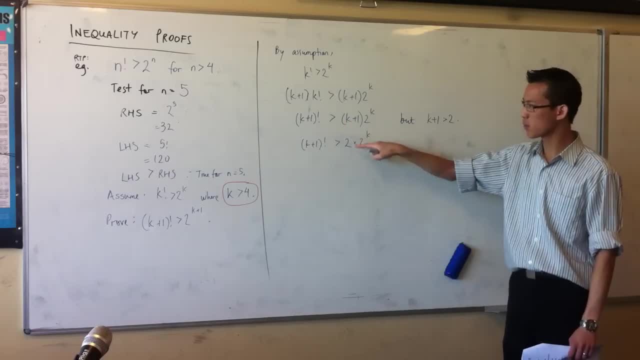 because it's like: oh, you're substituting stuff, but that's, k plus one is not equal to two. Okay, That's true, k plus one is better than two. Do you see why? you can just chop and chain things? 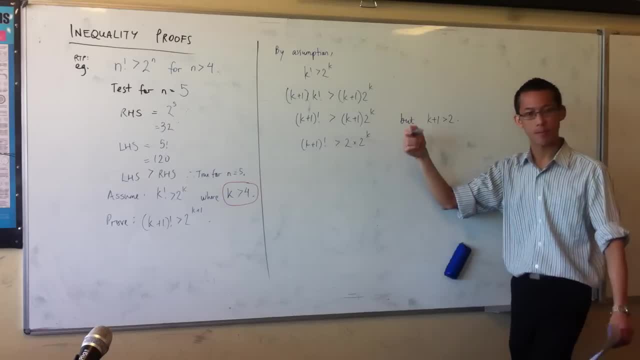 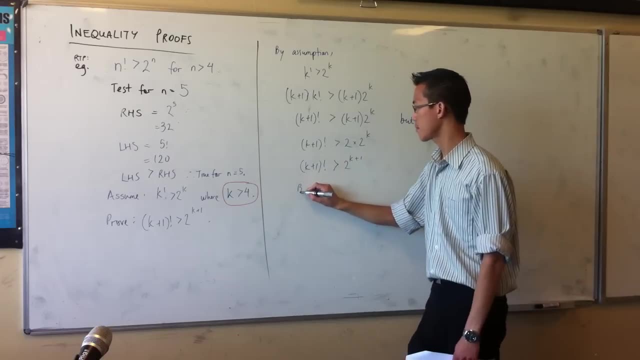 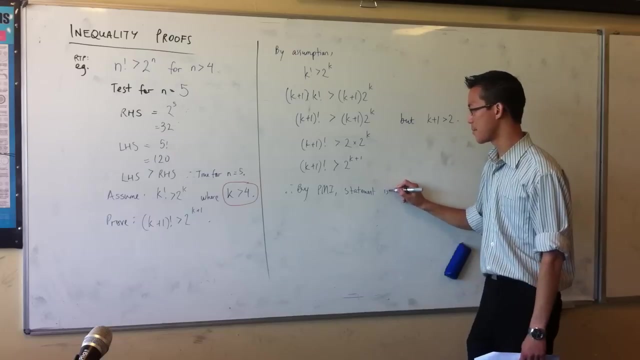 when you've got inequalities. Okay, And that's where my two to the k plus one is. Now, don't forget again the statement is true. for what? So you go back to your original question and they gave you the domain for it, right?